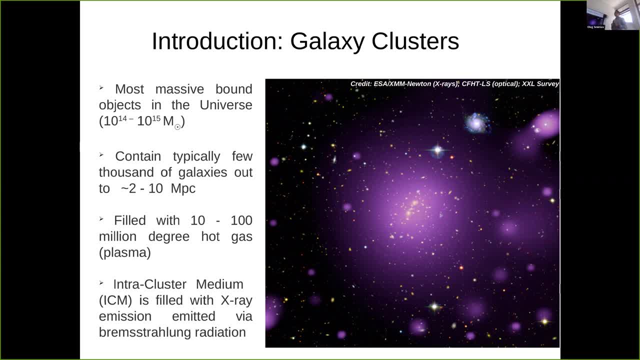 They typically contain from a few thousand of galaxies out to a radius of from 2 to 10 megaparsecs, and they are filled in with 10 to 100 million degree hot gas plasma. So we keep in mind that the intra-cluster medium is filled with X-ray emission, which is emitted via Bremsstrahlung radiation. 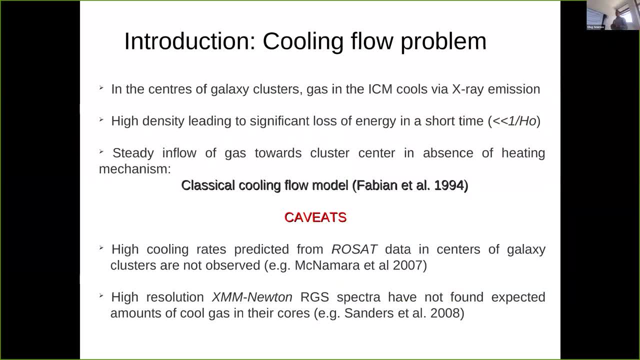 So this hence causes an expectation that in the center of galaxy clusters the gas in the intra-cluster medium will be cooled via X-ray emission. Well, the higher the density, it will lead to a significant loss of energy in a short time. So a steady inflow of gas. 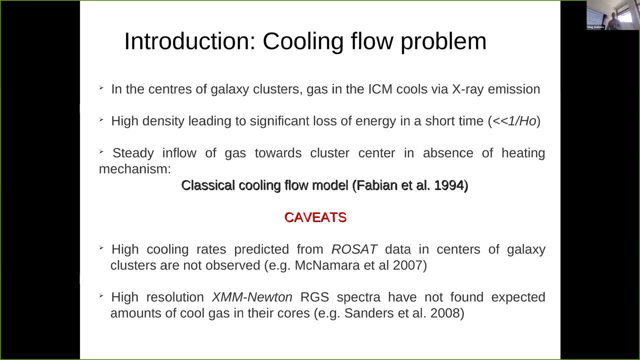 towards the center of the cluster in the absence of a heating mechanism should be observed, and this is the classical cooling flow models. but there are some problems. First of all, the high cooling rates that were predicted from ROSAC data in the centers of galaxy clusters are not observed. 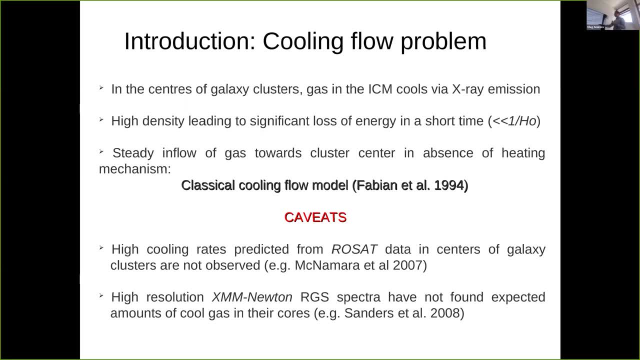 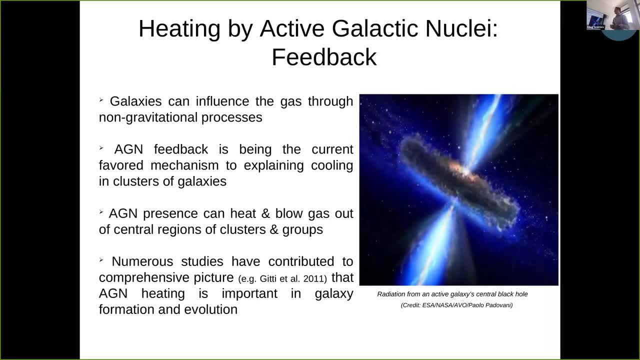 And secondly the high resolution XMM-Newton-RGS spectra. they have not found the expected amounts of cool gas in their cores, So this means that galaxies can influence the gas through non-gravitational processes. So Aegean feedback is currently being the 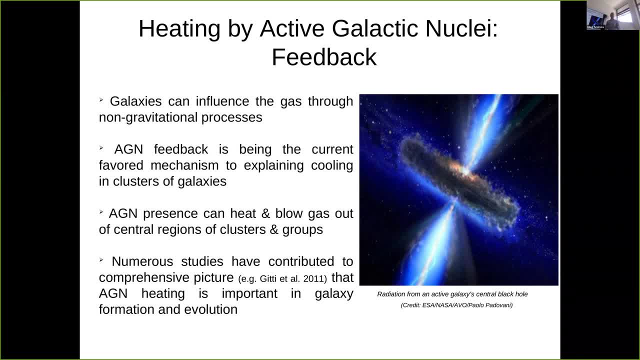 current favorite mechanism to explain cooling in clusters of galaxies: The Aegean presence can heat and blow the gas out of the central regions of the clusters and groups. Then there have been numerous studies that have contributed to a comprehensive picture that Aegean heating is. 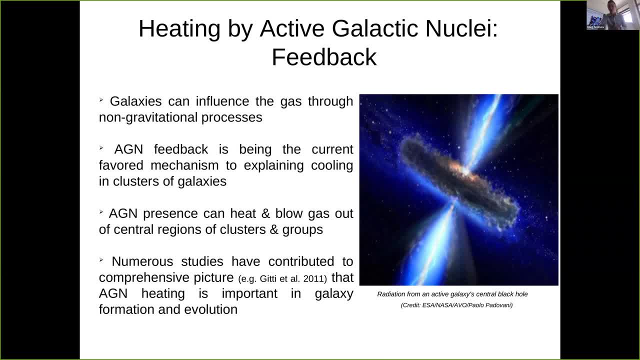 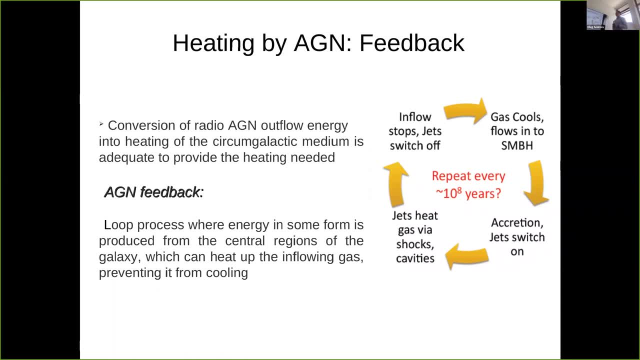 important in galaxy formation and evolution. So what is heating by Aegean? Basically, we have the conversion of the radio Aegean outflow energy into heating the circumgalactic medium, which is adequate enough to provide the heating needed. So by Aegean feedback. 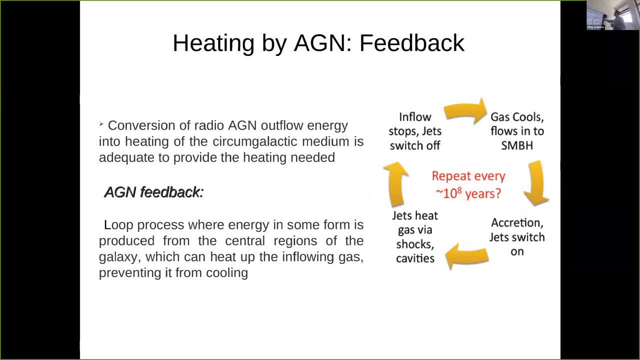 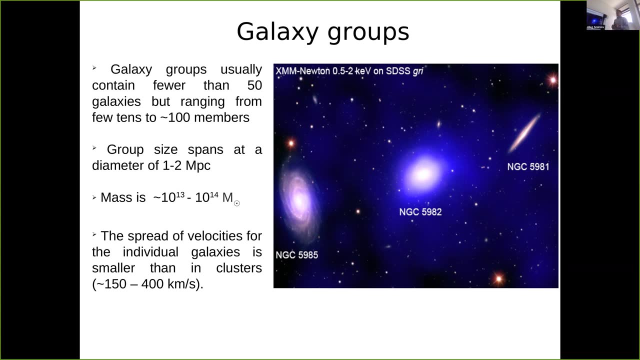 we mean the loop process, where energy in some kind of form is produced from the central regions of the galaxy and can heat up the inflowing gas, preventing it from cooling. And moving on now to galaxy groups. So they usually contain fewer than 50 group members, but 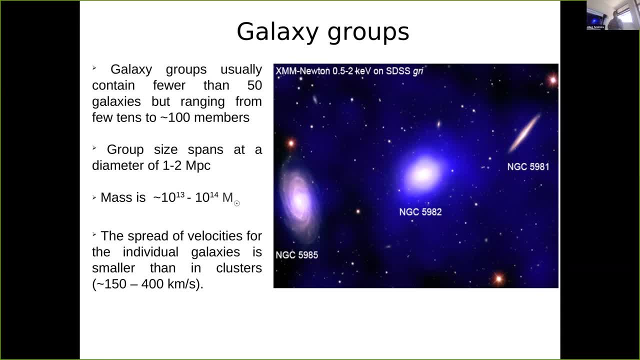 we have seen groups ranging from members between 10 to 100 members, And the group size is relatively smaller than in clusters. It spans from between one and two megaparsecs approximately, And their mass is between 10 to the 13 and 10 to the 14 solar masses. I mean 10 to the 13 and a. 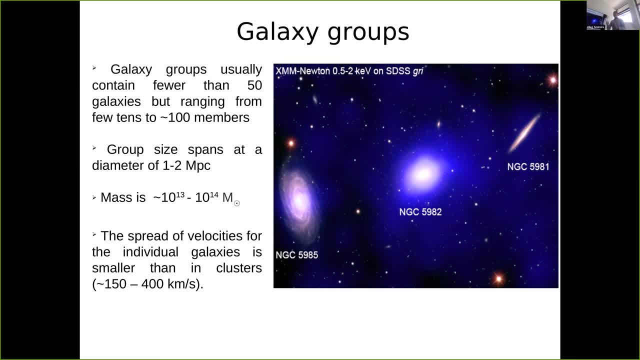 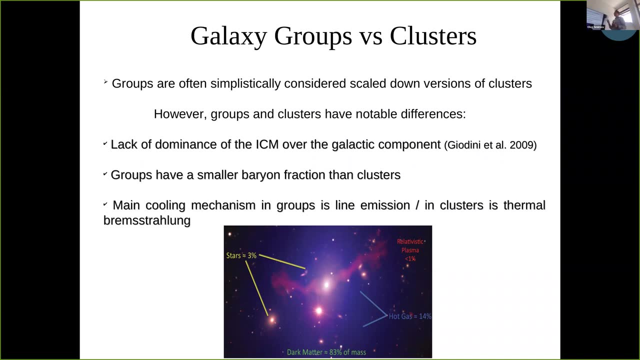 half and till 10 to the 14 is the gray area between the transition between groups and classes. The spread of velocities as well in galaxy groups, in the individual galaxies, is relatively smaller than in clusters, between 150 and 400 kilometers per second. And if we make a comparison between groups and classes, of course people 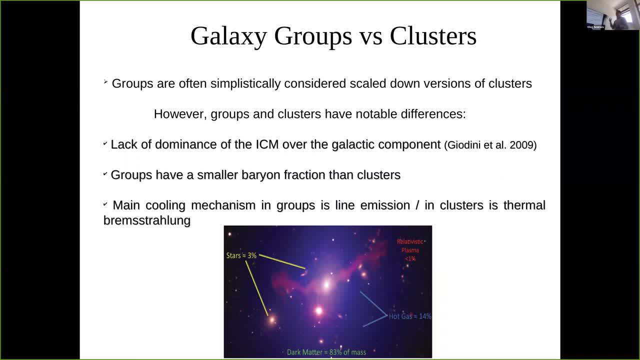 often symbolistically consider them as a scaled versions of groups, considered being considered as scaled down versions of clusters. However, they have notable differences. For example, galaxy groups: they lack the dominance of the interact group medium over the galactic component, which means that we have the interact cluster medium dominating the baryon content. in comparison, 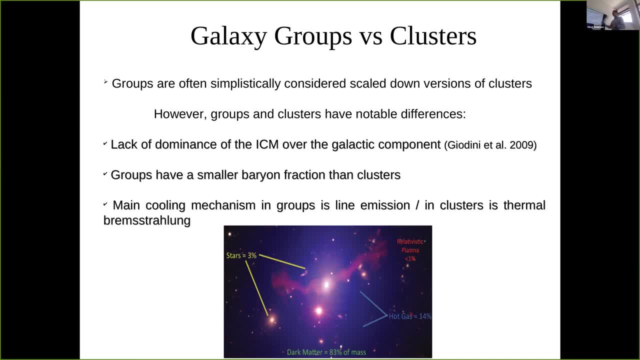 to the member galaxies, Whereas, on the other hand, in galaxy groups this might be even, or even the baryon budget in galaxy members can be higher than in the gas itself. In addition, groups have a smaller baryon fraction than in clusters And the main cooling mechanism in galaxy 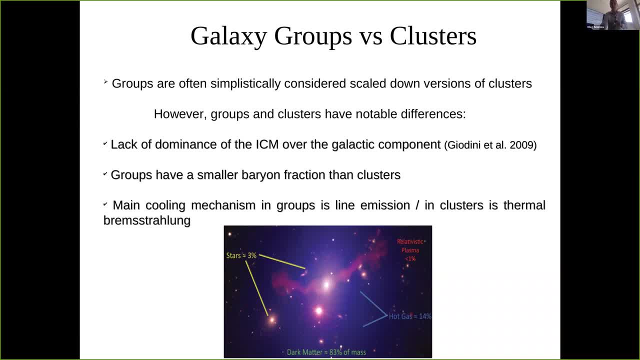 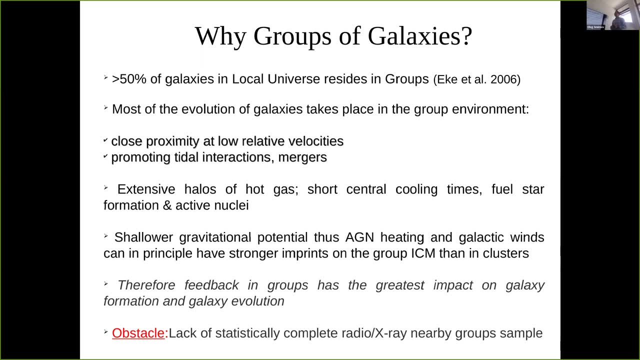 groups is line emission, whereas in clusters it is thermal brainstorming, as we just mentioned. So why should we then care about groups of galaxies? Well, more than half of the galaxies in the local universe resides in groups, And most of the evolution of the galaxies takes place in. 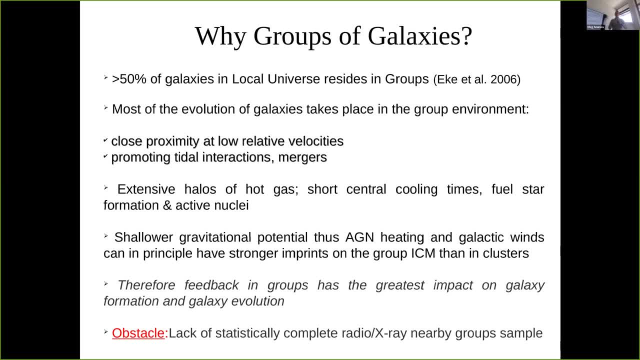 the group environment. All galaxies are into close proximity at the lower relative velocities, which promote standard interactions and mergers. Some of them, of course, also possess extensive halos of gas. They have short central cooling times and they can fuel star formation and active galactic. 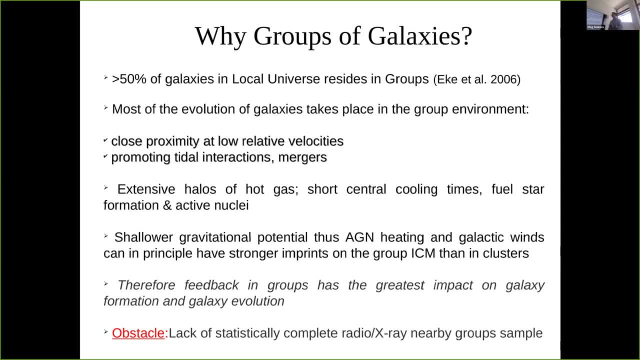 nuclei. In addition, they have shallower gravitational potential. thus the agent heating and galactic winds can, in principle, have stronger imprints in the galaxy group environment. Therefore, the agent feedback in groups has the greatest impact on galaxy evolution and formation. However, there is a problem. There is a lack of a statistically complete radio and x-ray nearby group. 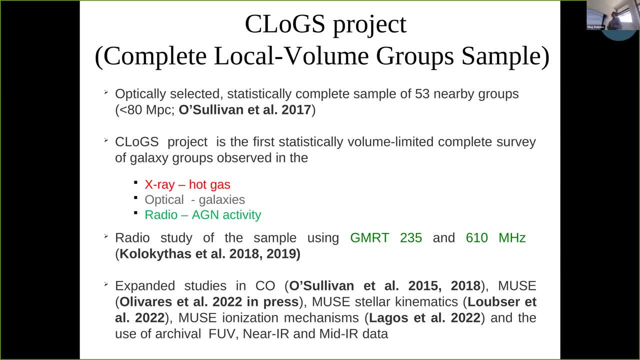 sample And in order to deal with this, we have started on embarked with the CLOGS project, which is an optically selected, statistically complete sample of 53 nearby groups in less than 80 megaparsecs, And the CLOGS project aims to be the first statistically 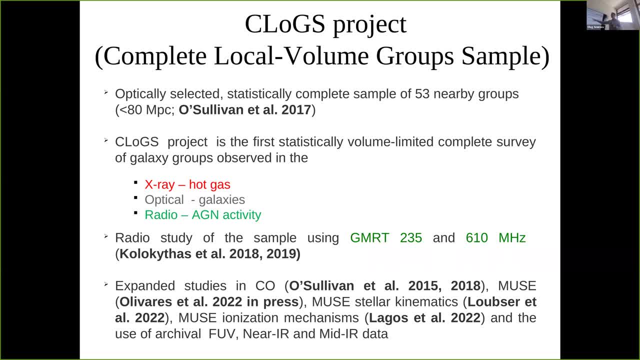 volume limited. complete sample of galaxy groups observed in the x-ray, optical and radio wavelengths. The radio study of the sample was performed in 2018-19 by myself using the GMRT-235 and 610 megahertz data, And so far we have expanded the studies with my 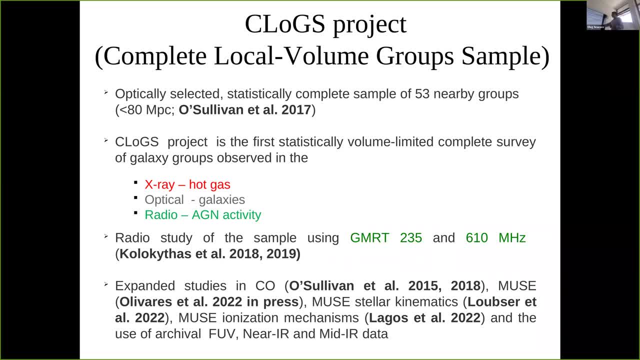 colleagues, Osalivan et al, into CO cold molecular gas and NEWS data optical from Olivares. stellar kinematics by Laubscher et al earlier this year. NEWS ionization mechanism by Lagos et al and, of course, the use of star formation indicators, which I will talk shortly. 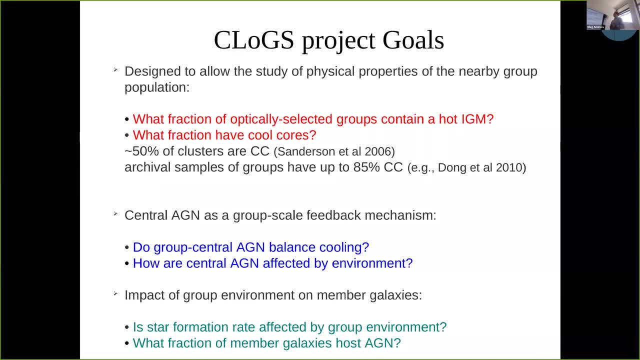 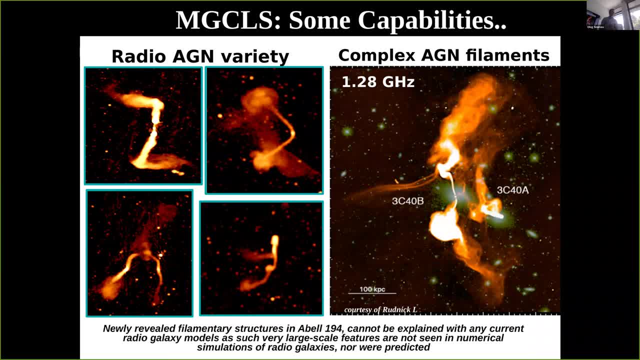 sorry, some of the projects that this, sorry, some of the projects that this, They get their revenge. I'm sorry, I'm sorry. There are actually populations in the 6th century, maybe back in the early 90s, or larger. 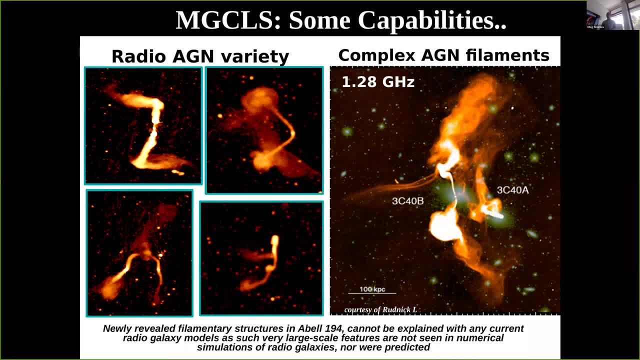 plus even lower. Oh yeah, yeah, I mean, there was one in Hogan et al, if I'm not mistaken, in 2015, and all Yes, And they get the similar detection rates for the central galaxies- yes, Above 80%, if I'm not mistaken, or 90% even, I think.